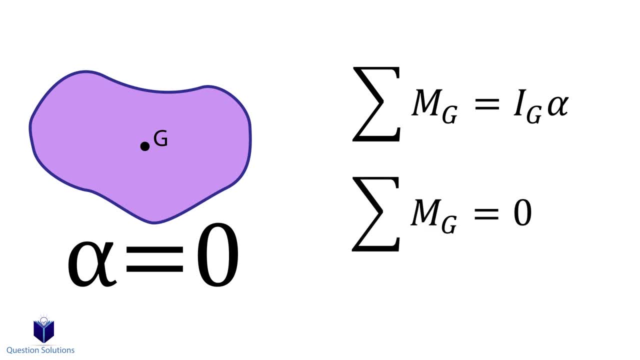 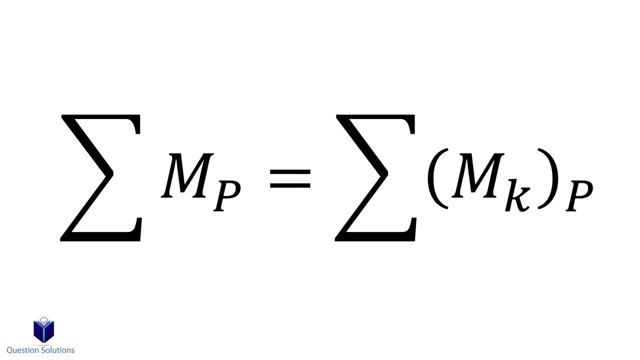 moment equation like this. You will see, when we do, examples on how to use this to solve for unknowns. There is also another equation tied to this moment equation. That's when we calculate the moment about a point other than the center of mass, Instead of picking. 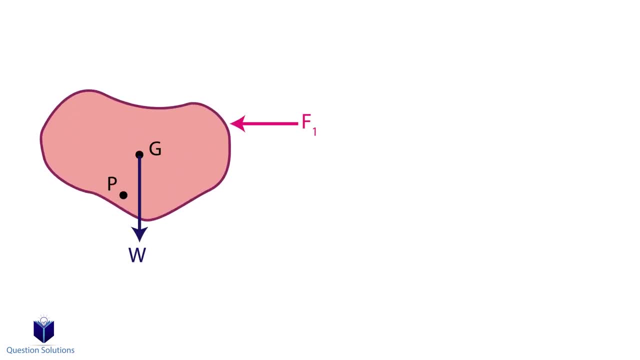 point G, which is our center of mass. let's say, we pick a point right here, We will label it point P To calculate the moment, we actually need to draw something called the kinetic diagram. To do so, we first pick the center of mass, Then we can draw. 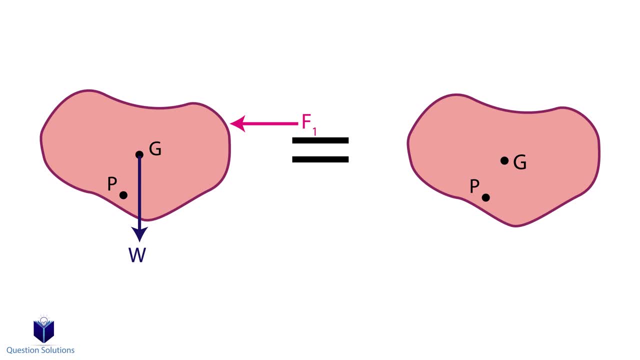 a vector to show the mass times acceleration the object would experience due to all the forces or moments affecting it. If the blob is going through curvilinear motion, then we can draw two vectors: that shows mass times, the normal acceleration, and mass times, the tangential acceleration. So a kinetic diagram for our blob would look like this: 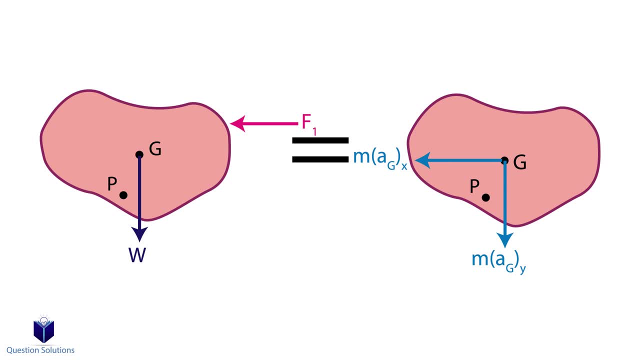 We have the mass of the blob multiplied by the acceleration. We show the mass times acceleration that occurs due to the sum of all the external forces that's affecting the object. The direction of the acceleration is assumed. Now to write our moment equation, we use the free body diagram for the left side and for the right side we use the kinetic. 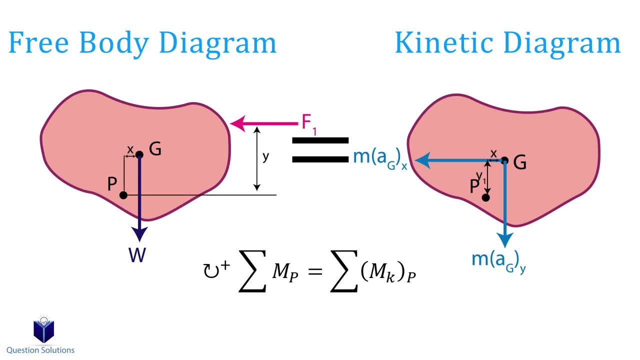 diagram. Remember that a moment is force times: the perpendicular distance to the point where we are calculating the moment at. So, for this example, our left side would look like this And the right side would be like this: Notice how the vector we drew at the center of mass. 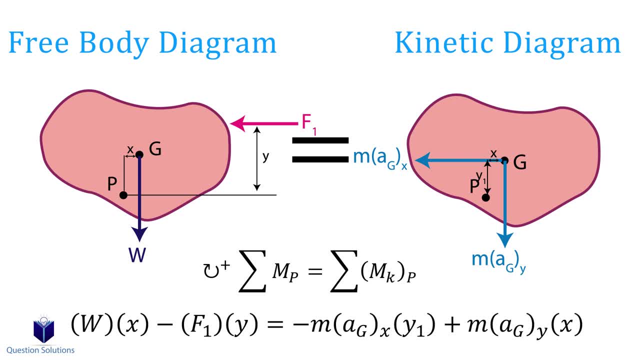 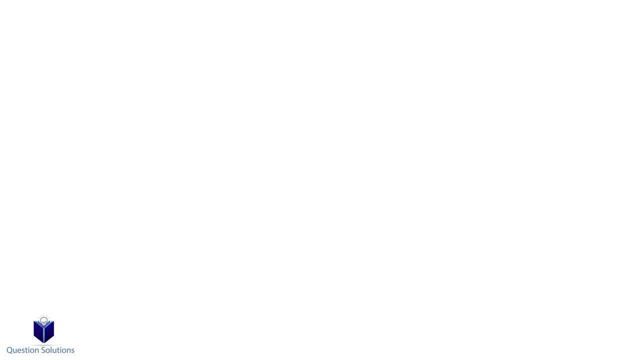 in the kinetic diagram is used to find the moment about point P. This might be a bit confusing right now, but after we go through examples it'll become much clearer. The first example will be very easy, without using any moment equations. In example number two: 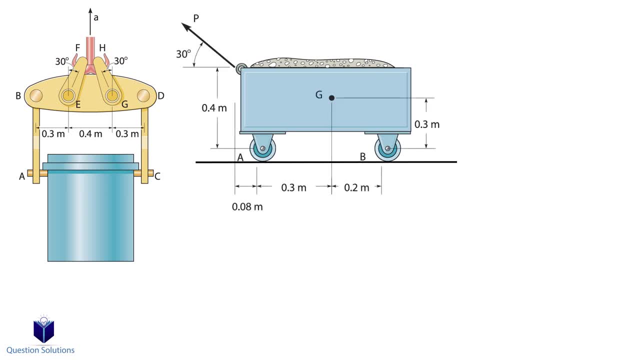 we will calculate the moment about the center of mass. For the third example, we will calculate the moment about a point other than the center of mass. We will look at how to use a kinetic diagram to solve the question. For the very last example, we will take a look at normal and tangential components. 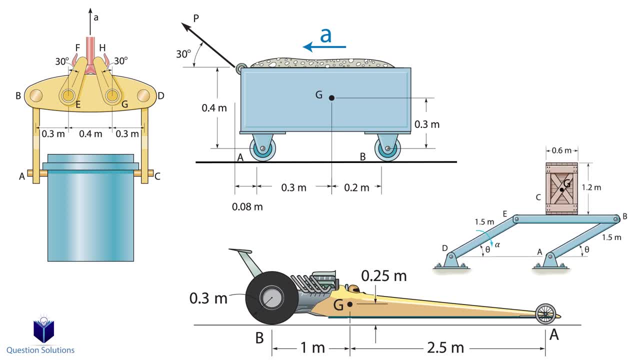 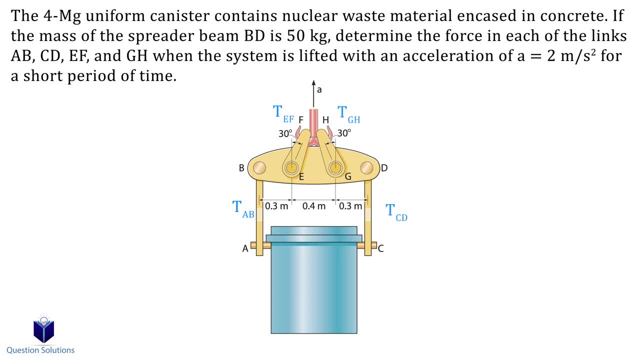 By the end, you should have a pretty good idea on how to solve the problems you will face. Let's take a look at this problem, where we need to find the force in the links AB, CD, EF and GH. First, let's draw a free body diagram of the canister: The canister. 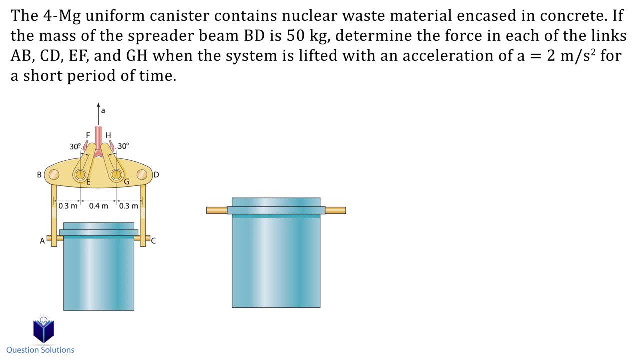 is held up by two links, AB and CD. Each will carry a force. The force affecting the canister would be weight, which would be downwards. Now we can write an equation of motion for the vertical forces, just for the canister. So we are ignoring. 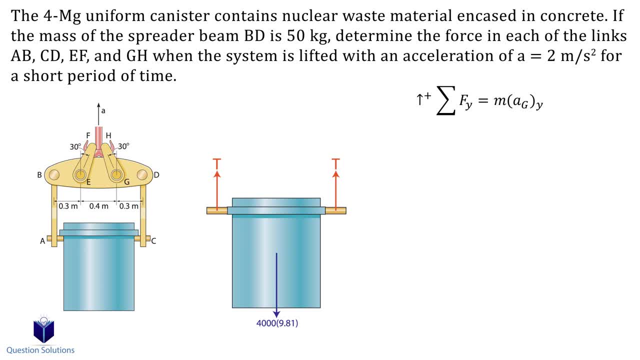 the weight of the beam, BD, We will pick up to be positive. So we have 2T, thus the two links holding the canister. Then we have the weight, so that's mass times the acceleration due to gravity, which is downwards, so that's negative. Then on the other side we have 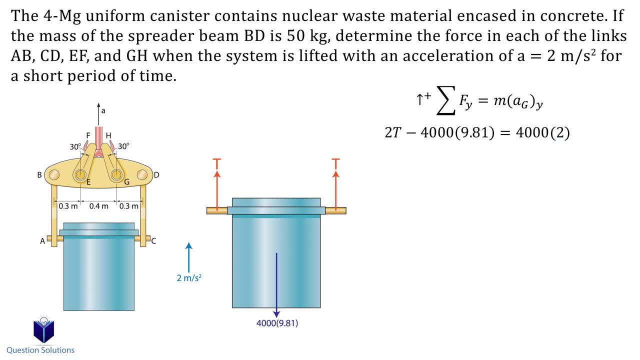 the mass of the canister multiplied by the acceleration. The question says it's an acceleration of 2 meters per second. squared upwards, We can solve for T, which gives us the force of each of the links AB and CD. Now let's consider the whole system, In other words, 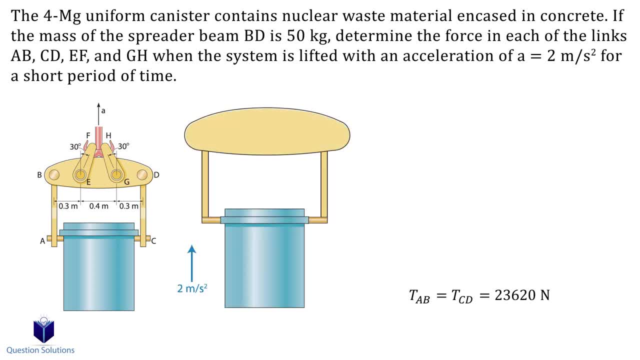 we're going to consider the beam that's on top. Let's draw another free body diagram. This time the forces that's holding the beam is at an angle of 30 degrees. We also have to consider two weights, one of the beam and one of the canister. Let's write: 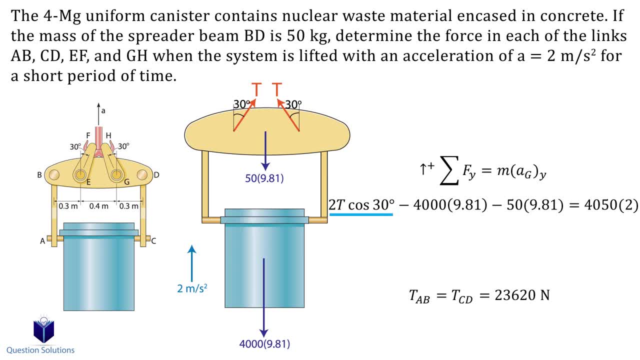 another equation of motion. So we have the y component of each force, We have the y component of each force, which is the force, so that's two forces. And then we have the weight of the canister and the weight of the beam, And that's equal to the mass of the whole system multiplied. 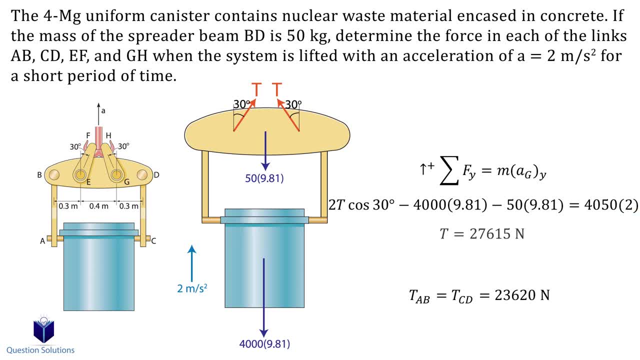 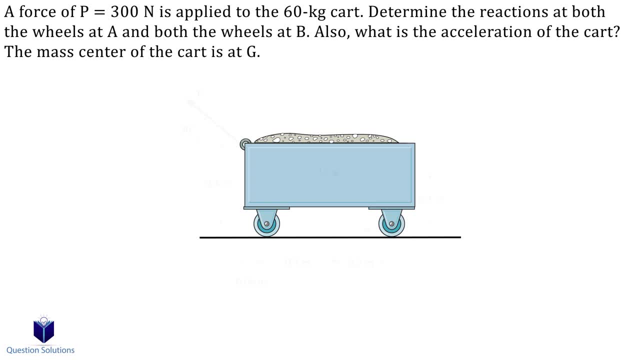 by the acceleration given to us. Solving gives us the forces in links EF and GH. Let's take a look at this question. We need to find the reactions at wheels A and B and we will also need to find the acceleration of the cart. First we will draw a free body. 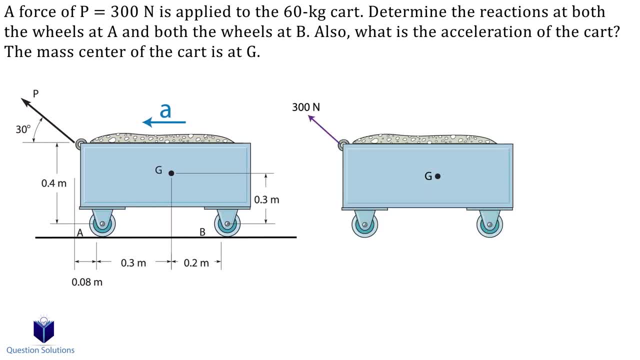 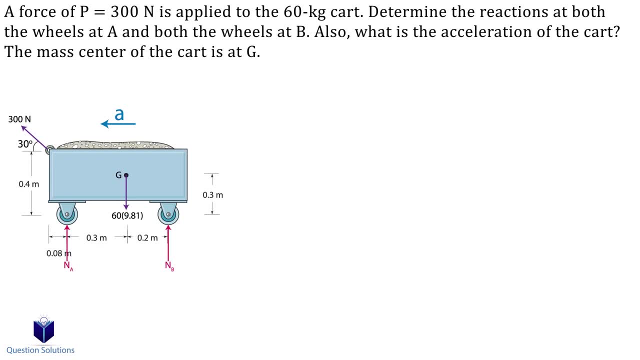 diagram of the cart like this. So we have the 300 Newton force, the weight and the normal reactions at wheels A and B. To figure out the acceleration, all we need to do is write an equation of motion for the horizontal forces and we will pick left to be positive. 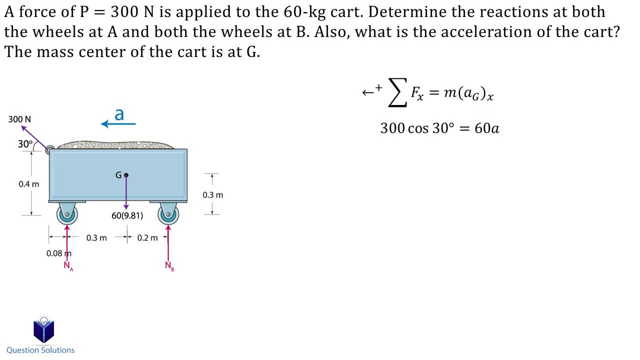 So we have the x component of force P, and that's equal to the mass of the cart multiplied by the acceleration in the x direction. Since the cart only moves along the horizontal axis, there won't be any acceleration upwards. We can solve the equation which gives us: 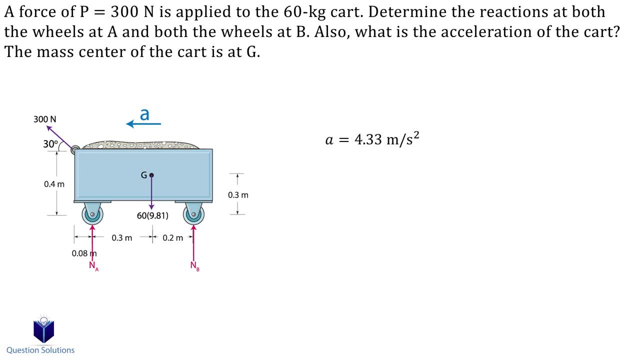 the acceleration. Solving the reactions at the wheels will require two equations. since we have two unknowns, NA and NB, The first equation will be for vertical forces. So we have the two reactions at the wheels and the y component of force P, and from that we subtract the weight On. 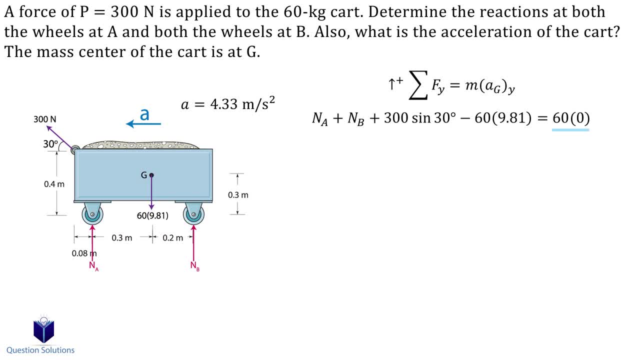 the other side we have the mass of the cart multiplied by the acceleration, but again the cart only moves in the horizontal direction, meaning it doesn't move up or down. So there is no acceleration in the vertical direction. Now we need another equation For this. we will write a moment equation about the mass. 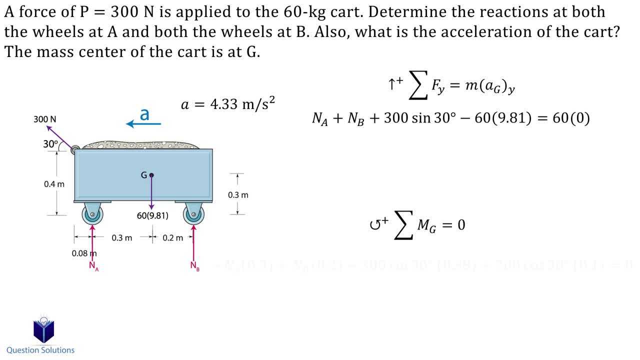 of center, point G, We will pick counterclockwise to be positive. Let's go through this equation, But first imagine that we pin this cart at point G so it can freely rotate about the said point. If we apply the reactions at A like this, we see that the cart would turn. 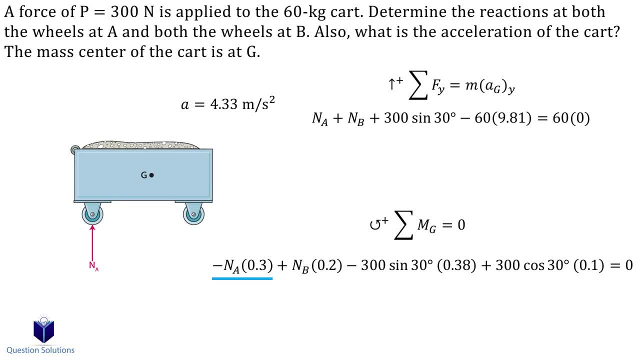 clockwise. So then the moment is negative, since we picked counterclockwise to be positive. Remember, moment is force times the perpendicular distance of the cart multiplied by the acceleration. So we have the distance of point A to point G. Then we have the reaction at B and we 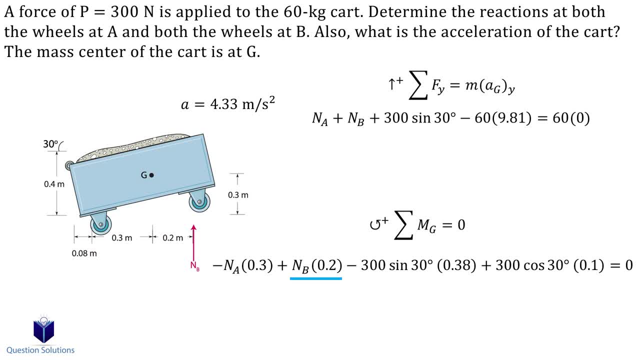 see that if we apply that force, the cart would spin counterclockwise. So it will be a positive moment and the distance is point 2 meters. Next we have the 300 Newton force, which we can break into two components like this: 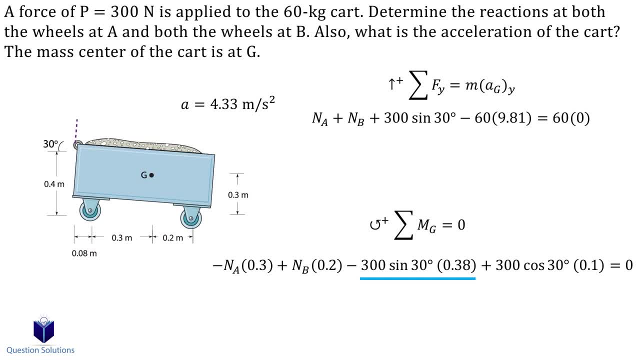 If we look at the vertical force, which is 300 sine 30 degrees, we see that the cart would spin clockwise, So that would be a negative moment. The distance is from where the force is being applied to the center, which is point 3 meters plus the point 08. 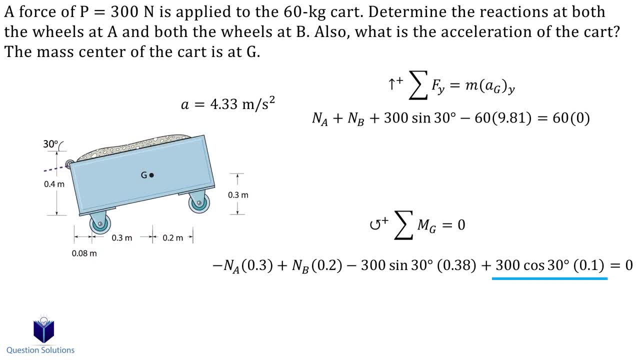 meters For the horizontal force, we see that the cart would spin counterclockwise, So that will be a positive moment. Since this is a horizontal force, we will consider the vertical distance to the mass of center, which means it's point 4 meters minus point 3 meters. 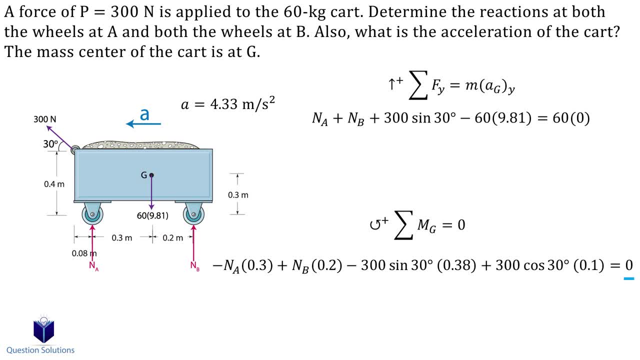 giving us point 1, meters. All of this is equal to zero, since the cart is in the middle of the cart and is not spinning and is only moving in the horizontal direction. We now have two equations with two unknowns. Solving them gives us the reactions at wheels. 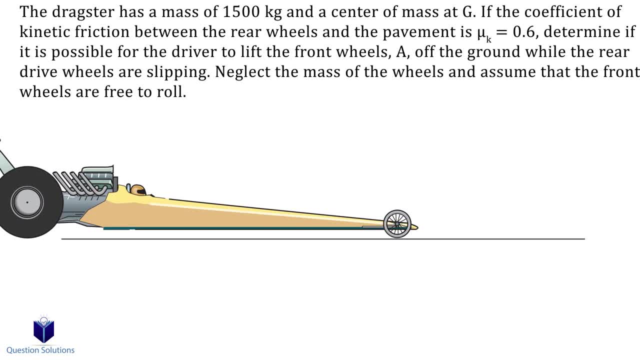 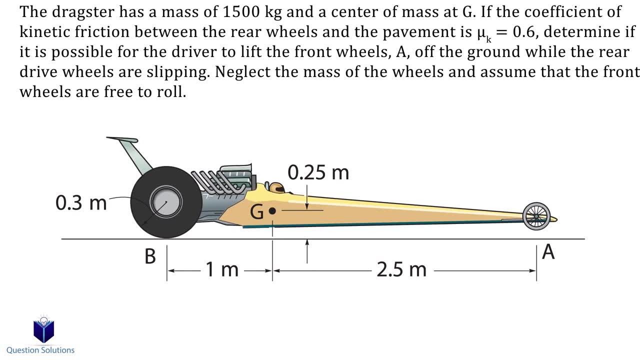 A and B. Let's take a look at this example where we actually write a moment equation where it's not above the center of mass. So in this question we need to show if it's possible for the front wheels of the cart to lift up while the rear drive wheels are slipping. 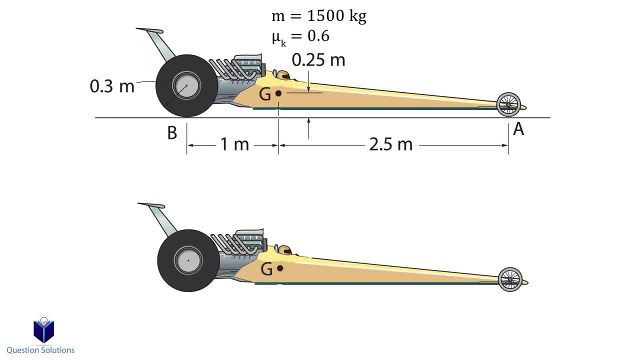 First we will draw a free body diagram. We have the weight, the normal force at the rear wheels, but from the question we know the front wheels are supposed to lift up, which means the normal force at the front wheels will be zero. Also, since the wheels are slipping, 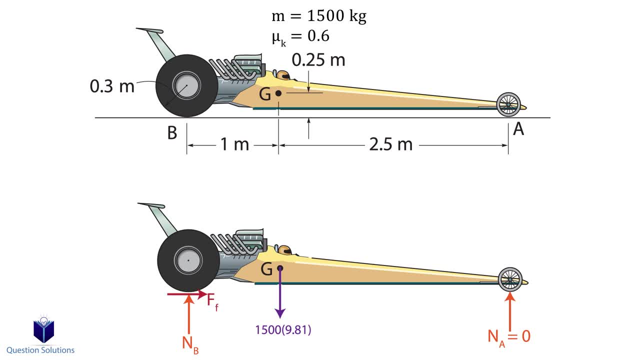 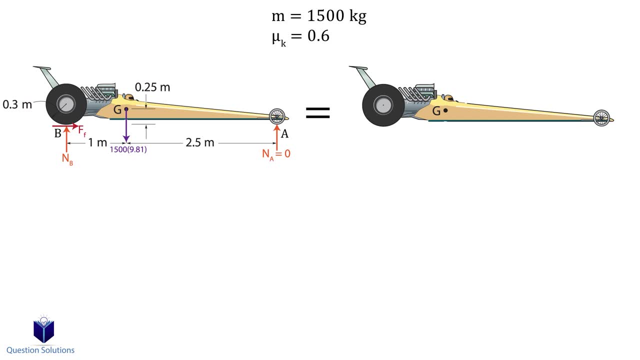 while rolling, the frictional force will be pointing to the right. Now we need to draw a kinetic diagram. So what that means is we need to use the center of mass given to us. Then we draw vectors that show the mass of the cart, times, the acceleration. 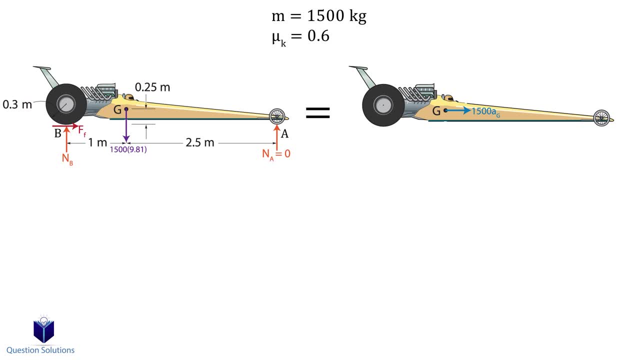 it would go through due to all the forces affecting it. In this case, the cart is only moving in the horizontal direction, so we'd have one vector pointing to the right. That would be 1500 times a. Using this, we can write a moment equation, but instead of writing it at the center of 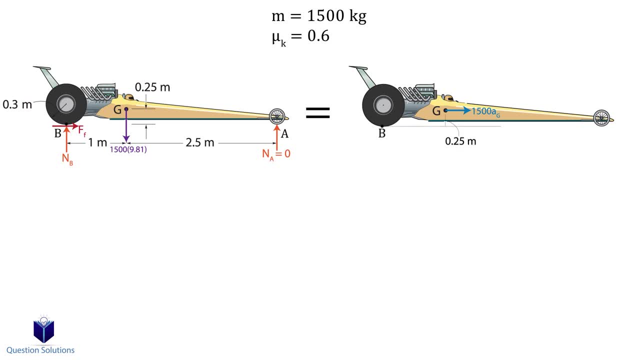 mass. we will write it at point B. Whenever we write a moment equation about a point, we can ignore the force being applied at that said point because it goes through the line of action. In simple terms, if we picked location A, then we ignore NA. And here, since we picked, 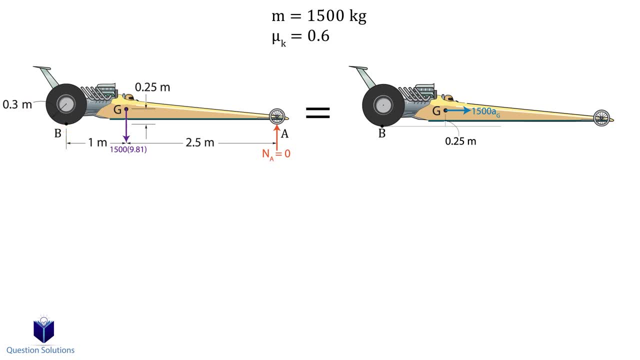 location B. we ignore NB and the frictional force which also goes through the line of action, So we will pick clockwise to be positive. You should also note that this moment equation is written with the free body diagram and the kinetic diagram, So on the left side. 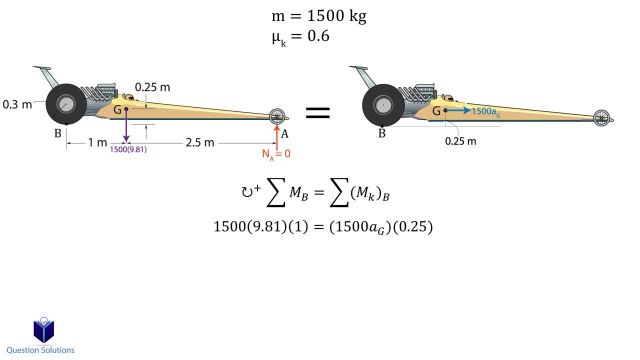 we have the mass times acceleration that causes a clockwise rotation, and the distance from the center of mass to point B is 1 meter. That's all the forces that will cause a moment for the free body diagram, since NA is 0.. Then on the other side, we look at the kinetic 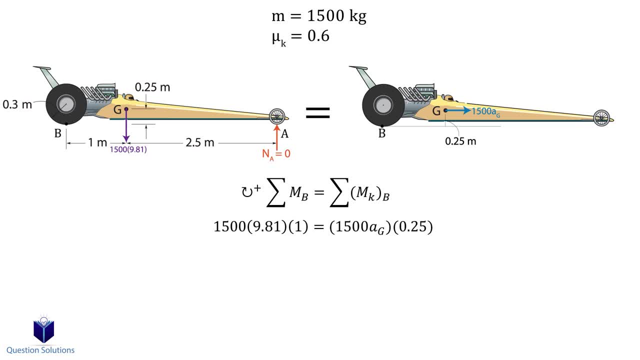 diagram We see that the mass times acceleration at the center would cause a clockwise rotation, so that'll be 1500A multiplied by the perpendicular distance to location B, which is 0.25 meters. We can solve for the acceleration. This is the acceleration at the center of mass of this. 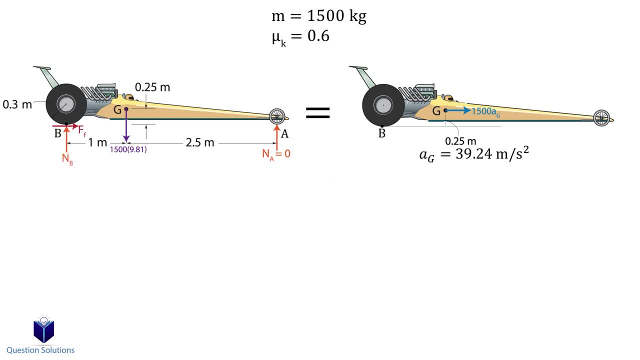 car. Next we can write our familiar equations of motion for horizontal and vertical forces. We have only the frictional force on the left side and on the right side we have mass times acceleration in the horizontal direction. Don't forget to plug in the acceleration we. 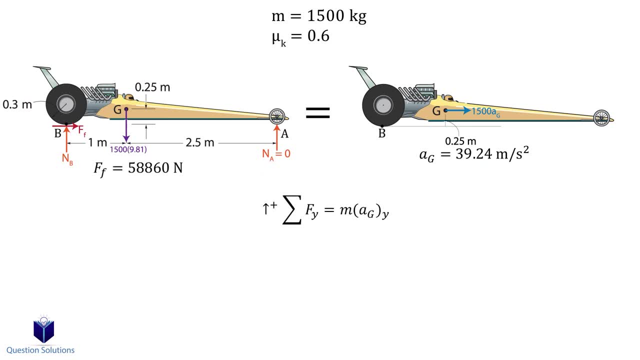 found To find NB. we can write an equation for the acceleration at the center of mass of this car. Next, we can write our familiar equations of motion for horizontal and vertical forces. We have NB and the weight on the left side and for the right side. remember the car. 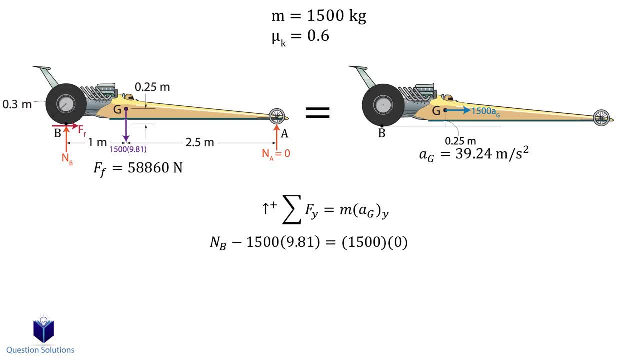 is only moving in the horizontal direction, so acceleration in the vertical direction is 0.. We can solve to get the normal force at B. So the question asks us if it's possible for the driver to lift up the front wheels. Well, let's calculate the maximum friction that's possible. Friction is a normal force. 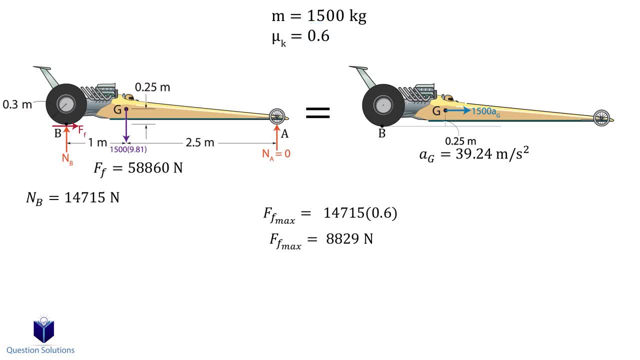 multiplied by the coefficient of friction. So this value we found tells us the maximum friction that the car can have with the coefficient of friction given to us. The value we found before tells us the required friction to lift the wheels up. In other words, when the wheels 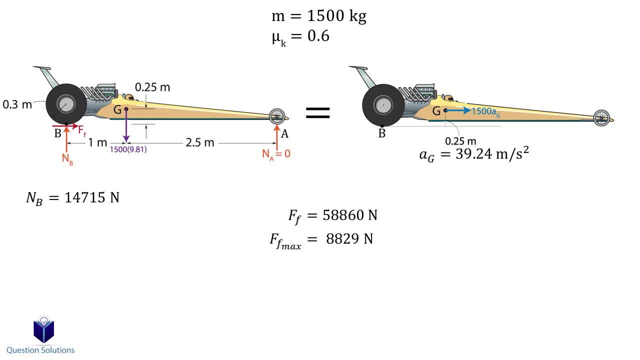 lift up, NA is 0, so we calculated the friction required to get NA to be 0. But with the coefficient of friction given to us, it's not possible to lift up the wheels, since we can't get the maximum friction to equal the friction required. 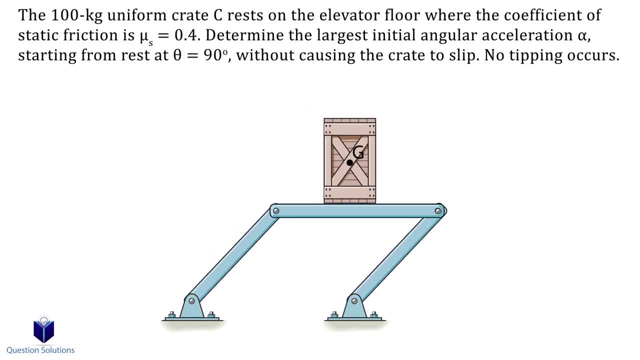 Let's take a look at one last question involving normal and tangential components. We need to find the largest initial angular acceleration before the box slips. In other words, how quickly can we rotate link DE before the box slips off? When we look at the diagram, we 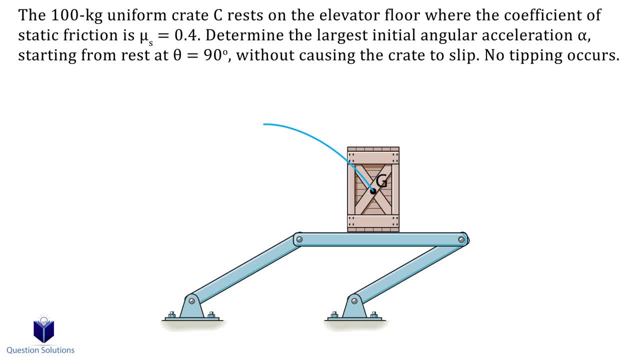 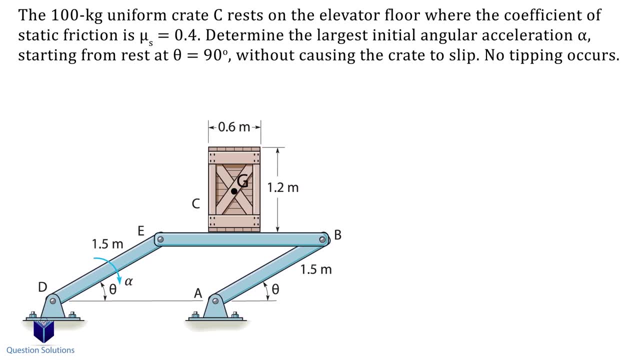 see that, as the link DE is rotating, the box on top would be traveling along a curvilinear path. So let's draw our free body diagram, but instead of using our normal x and y coordinate system, we will use the normal and tangential coordinate system. We have the weight, the 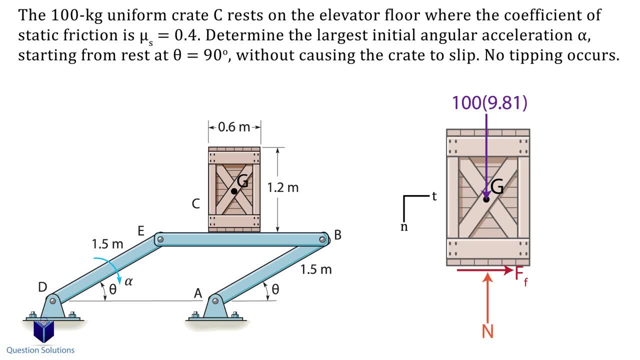 frictional force and the normal force. We will also draw the acceleration vectors, So the normal acceleration would be towards the center of the curve and the tangential acceleration would be straight ahead. Now we need to think about this problem. When theta equals 90 degrees, the angular velocity